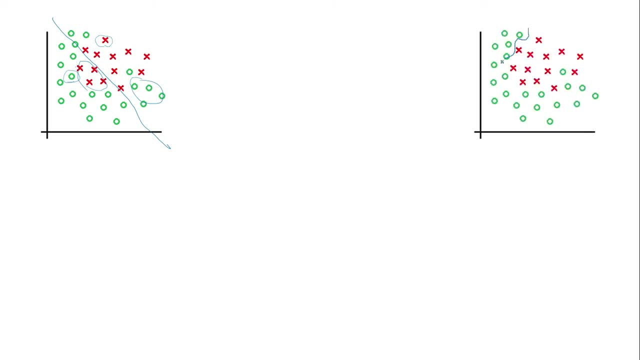 after certain tweaks to our model. our model fits so well to the data set and we achieve a very high training accuracy. Now if we use this model to plot the decision boundary on the test data set, then our decision boundary will fit something like this and we can. 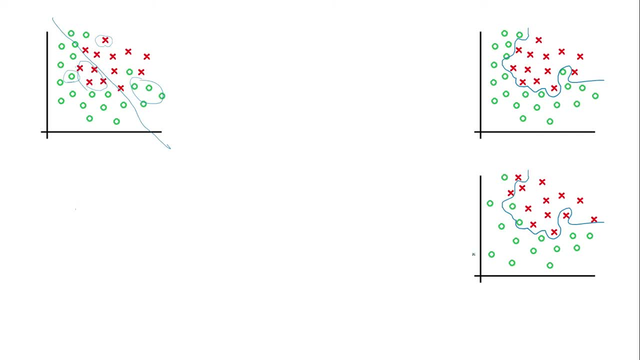 see that it is not performing well on the test data set. So in this case we have a high train accuracy but low test accuracy, and this condition is called overfitting, where our decision boundary is overfitting the test data set. Now, if we want to plot the decision boundary from a test data set, 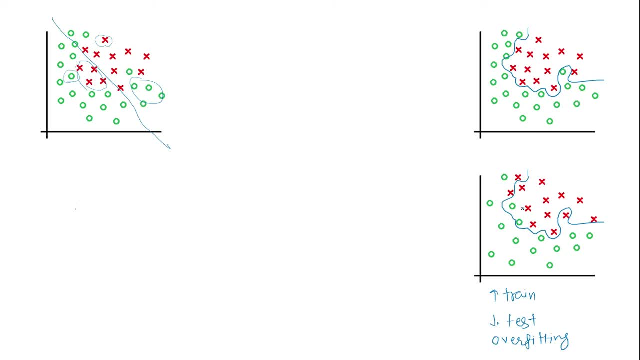 training data set and it is not performing that well in the test data set. Now, with this straight line, if we use this model and check the accuracy on the test data set, we can see that this is not performing that well either. So here we have low training data set and low test data set. 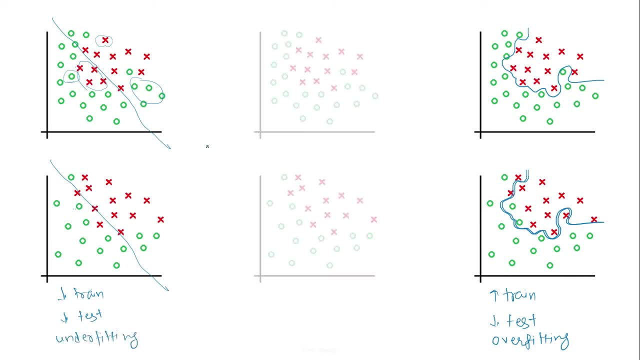 And this condition is called underfitting. What we are looking for is that: a decision boundary that fits well in both the test and the train data set. So we are looking for a high train and high test accuracy. When we have low training and the low test accuracy, we call this condition as high bias. 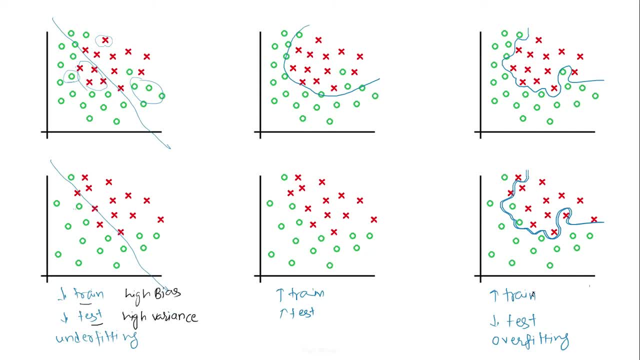 and high variance problem. And when we have a high train accuracy but low test accuracy, we call this problem as low bias but high variance, And when both the accuracies are high, we call it as a low bias and low variance. So how do we achieve this low bias and low variance in our model? 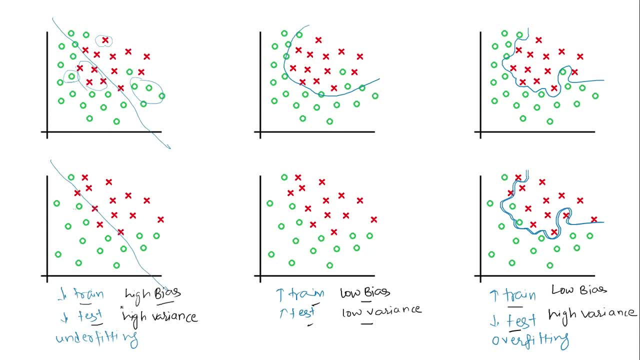 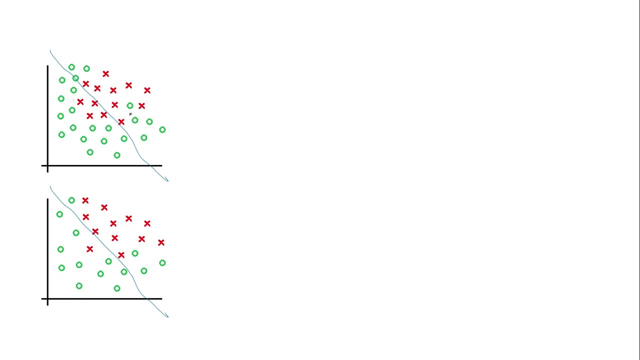 We can first start by improving our model to remove the bias and having the high train accuracy, and then making our model to have a high test accuracy as well. So let us start by first solving the underfitting problem. In case of an underfitting, it is very likely that our model is not very complex, but we 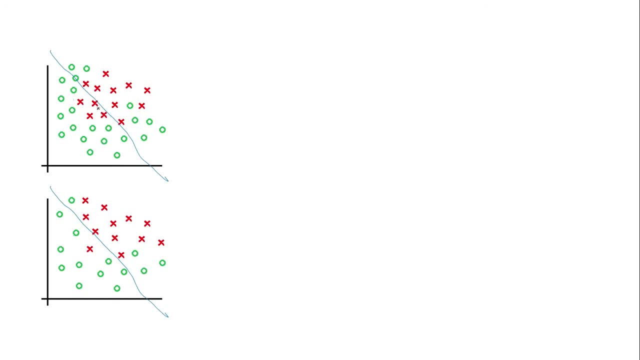 are using a very simple model. Since the model is not very complex, it is not able to recognize the complex features that are present in the data set. So one thing that we can do to overcome the underfitting problem is to use a complex model. 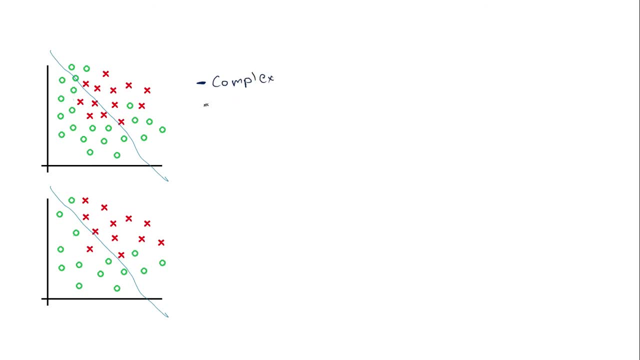 And if we are, let's say, using the neural network, then the way we can increase the complexity is by adding more number of hidden layers and more number of neurons in the hidden layers, And it can also be possible that the model was learning well, but we stopped halfway. 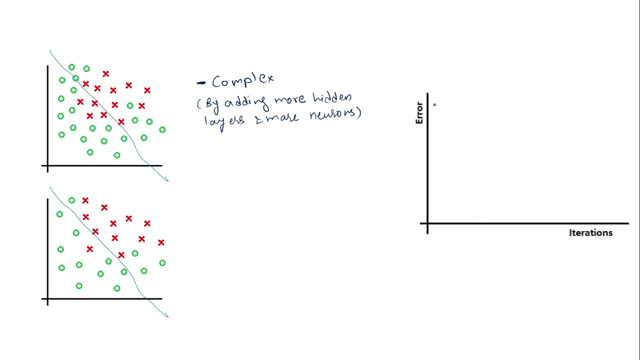 through the training. So if, when we plot the graph of the cost or the error versus iteration, it looks something like this for training data set, And if we stop the training process halfway through, then we can see that we can have a very high error in the train data set and thus the underfitting problem. 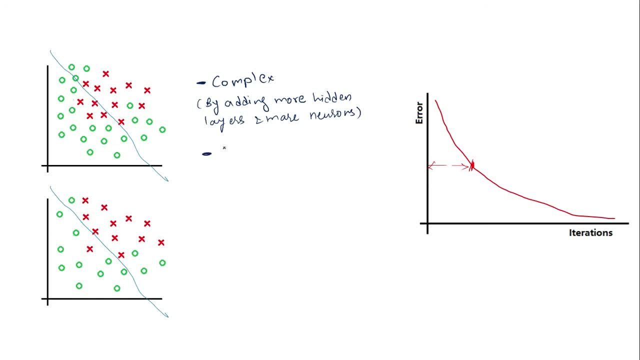 So the another way to overcome the underfitting is by training the model longer. So by trying these two methods it should solve our underfitting problem. but it is possible that we might end up having the overfitting problem. And if we plot the graph of the error versus the iteration for the test data set, it looks. 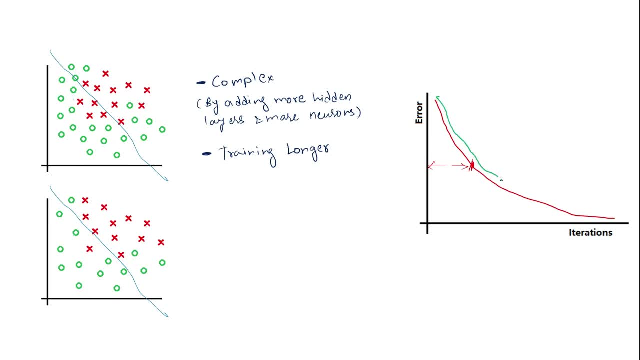 something like this, where it first decreases, but after a certain point it starts increasing. So we want a middle ground where we can have both the high test data set and the overfitting test accuracy, as well as the high training accuracy. So let us find the ways how we can solve the overfitting problem. 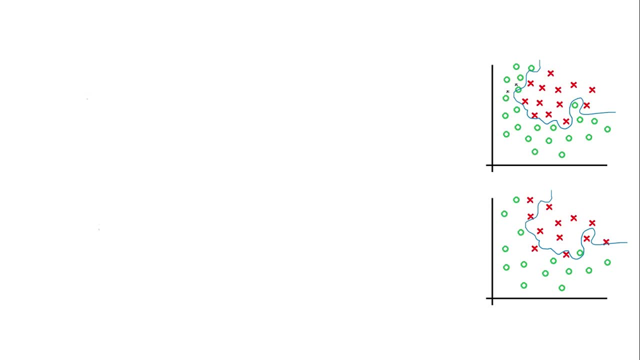 The overfitting is most likely to occur if we have a very small data set. If we have a small data set, then our model can quickly recognize the features and the patterns in this data set and can highly overfit it, And thus it will have challenge making the predictions for the test data set. 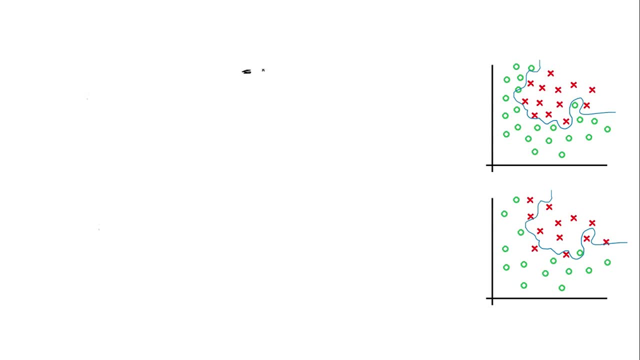 So a way in which we can overfitting The overfitting is by increasing the size of the training data set. But let's say, if we have the limited amount of data or the data is expensive, then how will we increase our training data set? 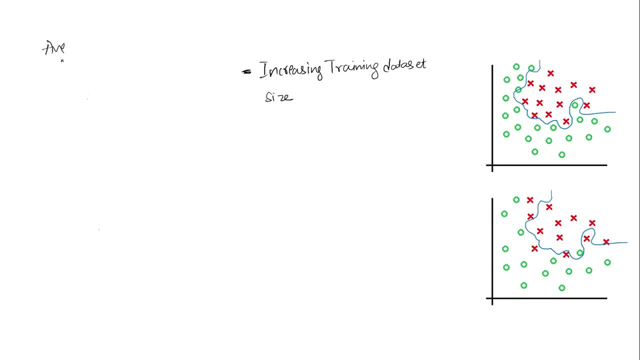 So the one way we can do this is by data augmentation, and data augmentation is a technique in which we produce new data from the existing data. For example, let's say we have the, we are dealing with the images of the cat, And if we flip this image or we take a mirror image of this image, this will still be a